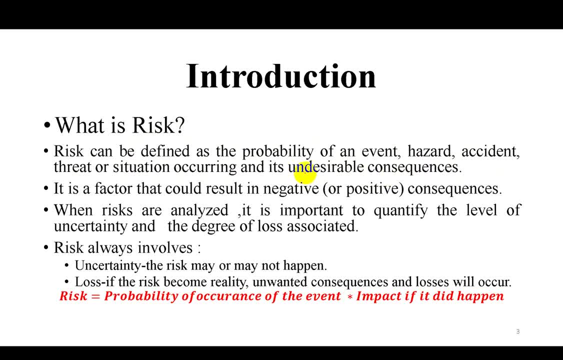 What does a general dictionary meaning of risk mean? We have any undesirable consequence, For example, any undesirable event, hazard, accident, threat or situation which may cause an undesirable effect on our normal routine. we call it risk. Risk is a factor that could result in a negative or positive consequence. 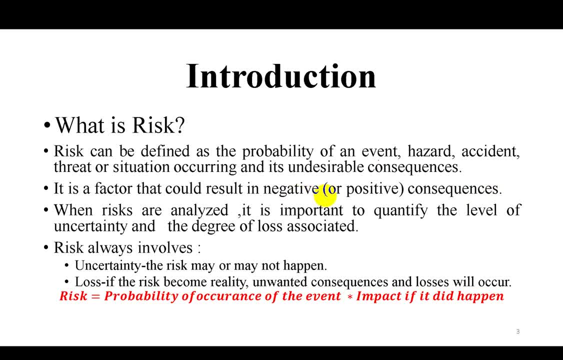 Generally the event which has a negative consequence or negative effect on it. we call it risk. When risks are analyzed, it is important to quantify the level of the uncertainty and degree of the loss associated with it. Generally, what is risk? It is a probabilistic event. 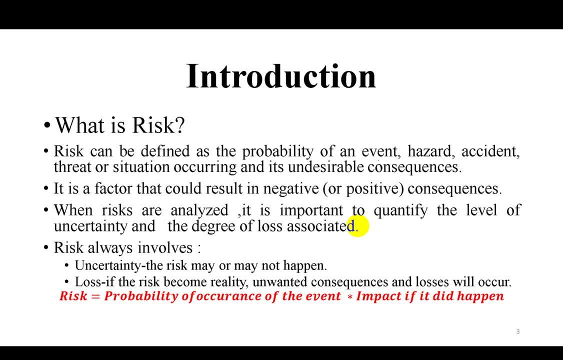 It is not necessary to have any risk. Whenever we identify risk, we do not know two things about it. First, what is the probability of happening that event means uncertainty? That quantifies the level of uncertainty. Second, what is the probability of the risk of uncertainty and the overall loss that is being degraded by it? how much does it impact our project? 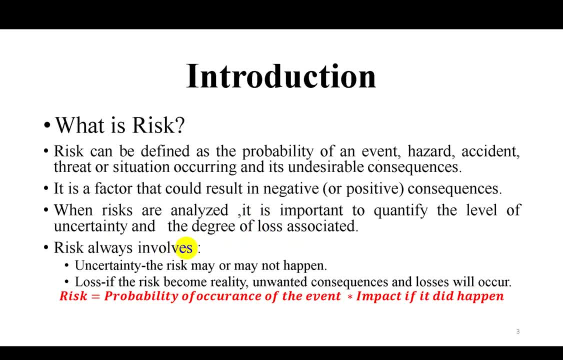 That is important for the risk. Risk always involves, as we have discussed, two things in the risk. one is uncertainty. uncertainty means the risk may or may not happen, It can be a risk or not. And the second is loss. If the risk happens, if the risk becomes reality, then the risk may or may not happen. 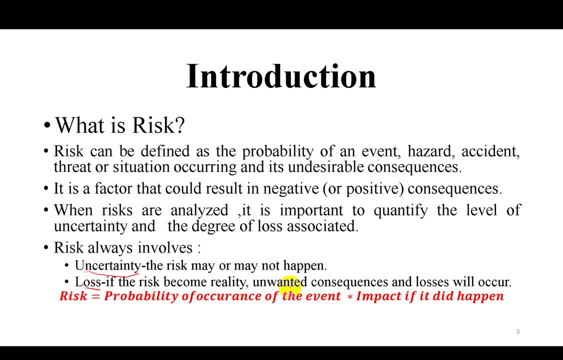 If the risk happens, if the risk becomes reality, then the risk may or may not happen. So that is the probability of a loss, And the third is probability of that event And this will offer us an indication of the risk. So how much will our system be affected by the probability of a loss? 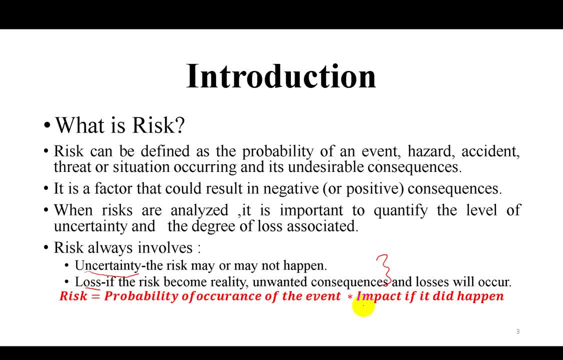 These two things are important for the risk analysis. So what is the risk? Risk is probability of occurrence of that event into impact. if it happened, If an event is happening, if there is a risk event, then how much will the risk be affected? 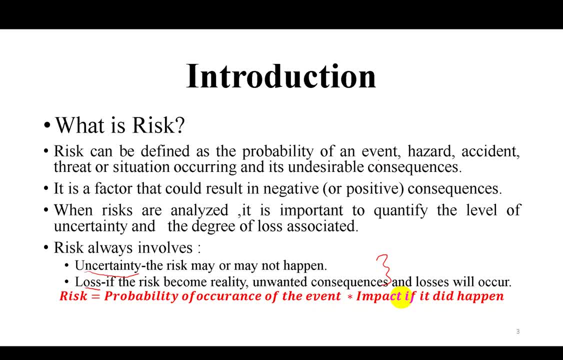 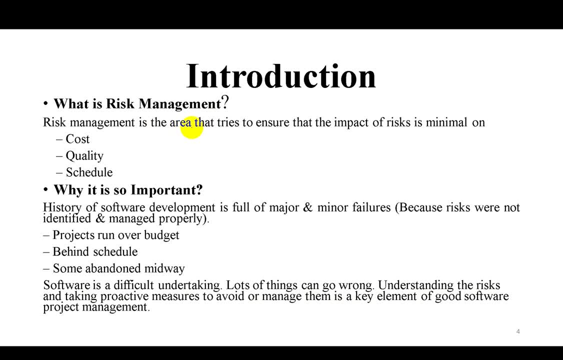 The multiplication of both of these things is known as the risk. What is risk management? Risk management is the relation between the creator and the resultant. And what is risk management? Risk management is the area which tries to ensure that impact of the risk is minimal. 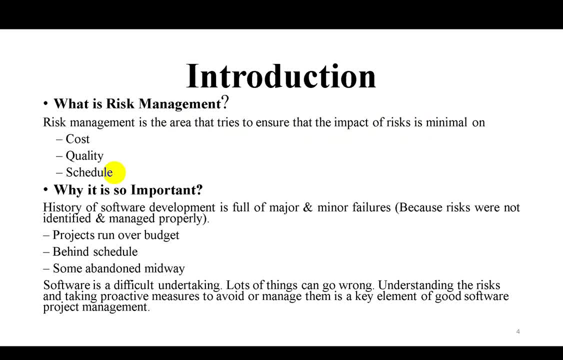 on cost, quality and schedule. Risk management is an activity by which we reduce or minimize the impact of risk on cost, quality and schedule. That is known as the risk management And why the risk management is so important. History of software development is full of major and minor failures. 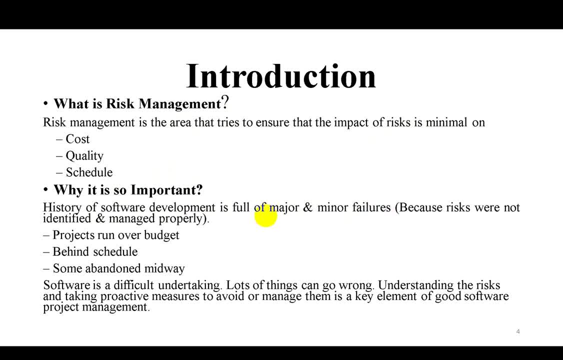 For example, we have a history that many of our big projects fail because risks were not identified and managed properly, And the main reason for their failure was that the risk was not properly identified and managed. What happened because of this? If we do not identify the risk and do not manage it, then the project runs over-budgeted. 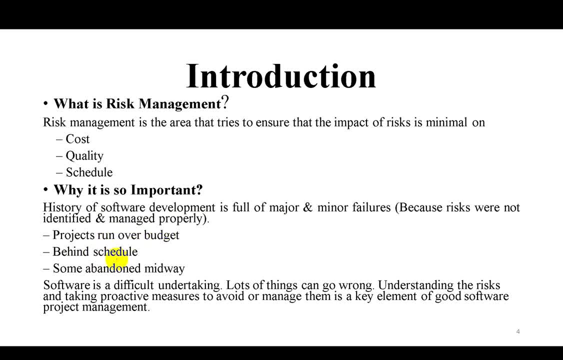 The project becomes over-budgeted, Behind the schedule, the schedule runs behind it Some abundant midway and sometimes we have to leave the project in between. Software is difficult undertaking Loads of things can go wrong. Understanding the risk and taking proactive measures to avoid and manage them is the key. 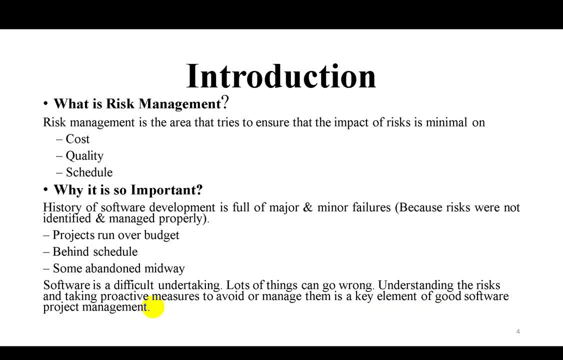 element of a good software project management. Software is an intangible product. Intangible is an image that we cannot see. It is in the form of a project, lines of code or software If we do not understand the risks in a project management and take proactive action for them. 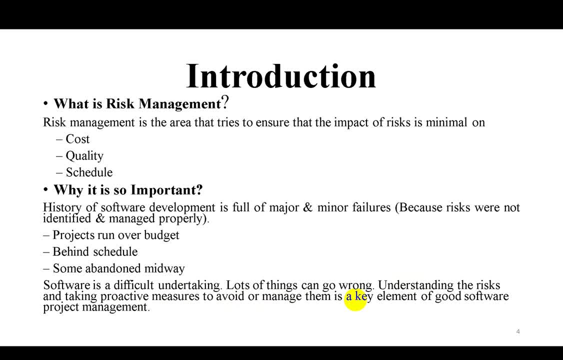 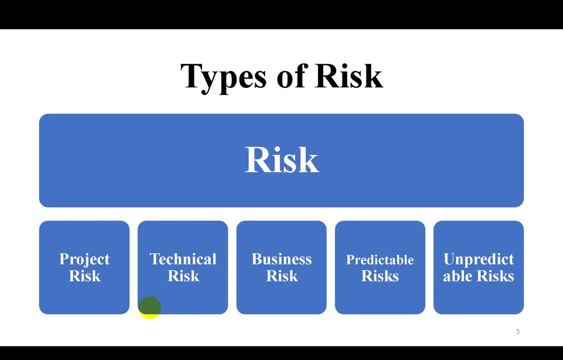 so that we do not have the risk, or if its effect is minimal, then what will we have? That is a good quality of a good software project. Now we will discuss about what are the types of the risks. The risks are divided into different categories. 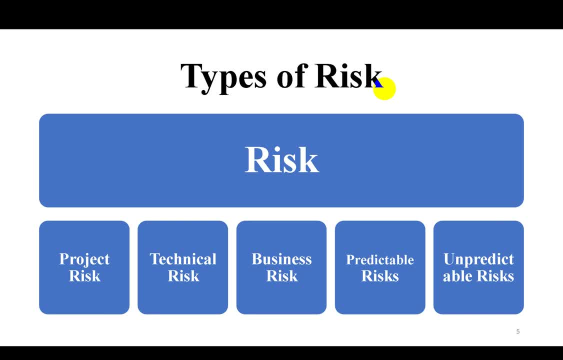 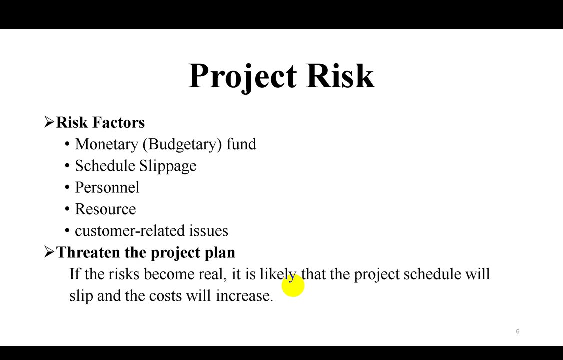 Here we will talk about these five categories. First is the risk related to the project. Second one is the technical risk. Third one is the business risk, Fourth one is the predictable risk And fifth one is the unpredictable risks. What is the project risk? 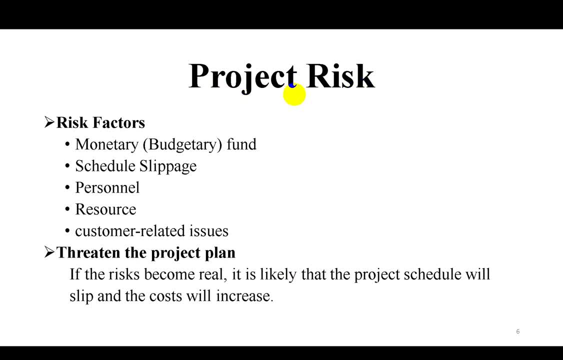 What is the project risk? What is the name of the project? What is the project risk? What is the risk that affects our overall project? The factors of the project risk are the monetary or budgetary fund, That is, we have an over budgeted budget. 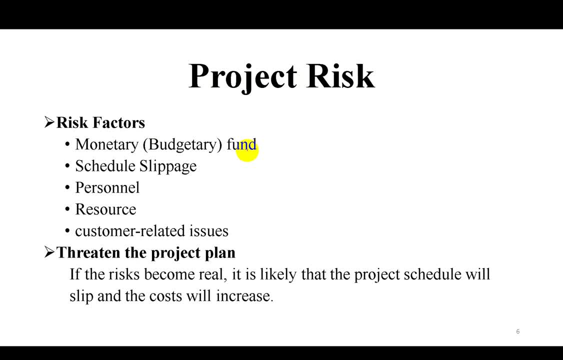 Or we had to cut the budget in the middle due to unavoidable circumstances. Second one is the schedule slippage, That is, our schedule is slipping, That is, it is moving backwards due to some factors. Personal- Personal means the software team, the persons attached to develop the software. 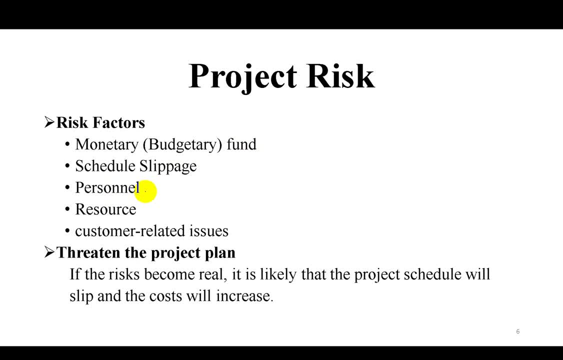 The factors related to that. What has happened to them? Some of the team members have left us Resources. Resources will include physical resources and practical resources. Whatever resources we need to complete that project. The factors related to that. Next one is the customer related issues. 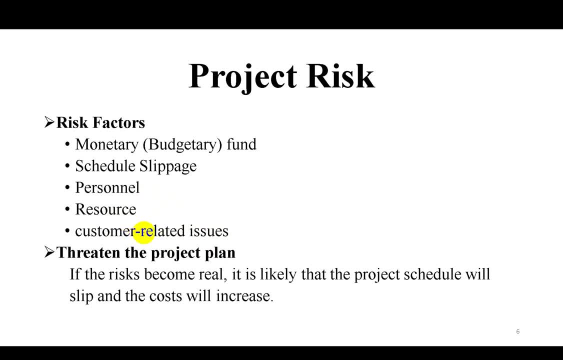 What are the issues related to the customer? What are the risk factors related to the customer? The risk factors are so much that it will be counted as a risk to the project, And what will be the effect of those risks? These can affect directly the project plan. 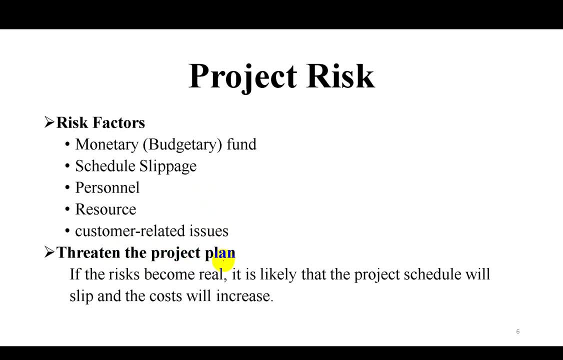 The planning of the project directly gets affected by these. If the risks become real- And if these risks become real- Then it is likely that the project schedule will be slipped and the cost will increase, Which is the major drawback of any software project process. 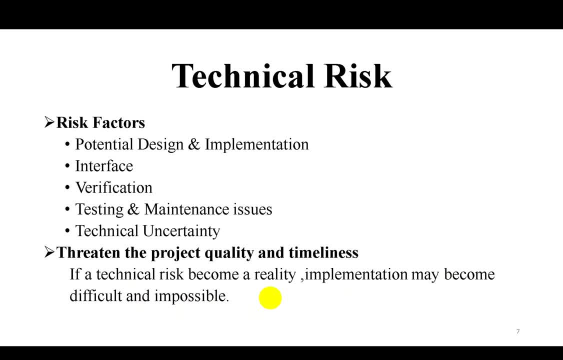 Second one is the cost. The second type of risk is the technical risk, which plays a major role in the technical risk Potential design and implementation. The risk involved in the design and implementation of the software project is known as the potential design and implementation related technical risk. 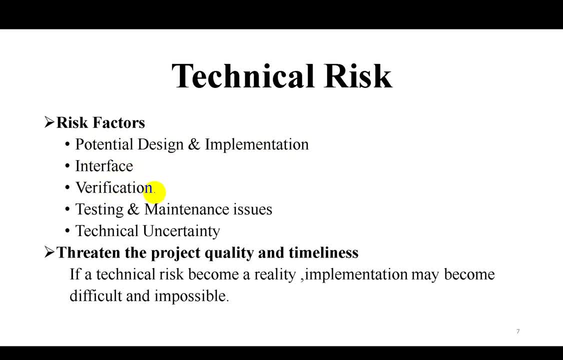 The second type is interface risk. The third type is verification. The fourth type is testing and maintenance risk. The fifth type is technical uncertainty. These risks can affect the project quality and the timeliness. Because of this, the quality of the project can be affected. 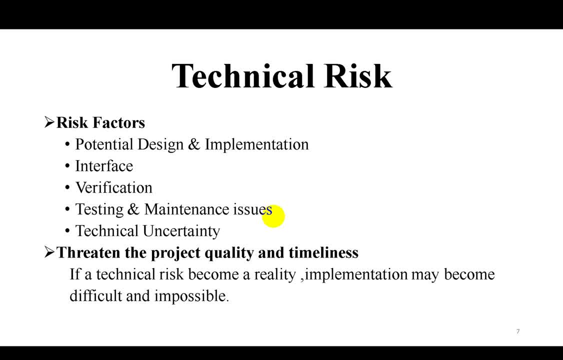 it can be degraded and the timeliness can also be affected. This means that the project can be delayed, Scheduled slippage can happen again. If the technical risk becomes reality, then the implementation may become difficult and even sometimes impossible. So the biggest technical risk related to this is that our implementation can be difficult and even sometimes impossible. 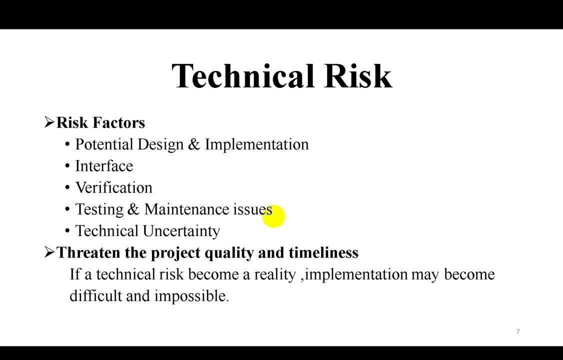 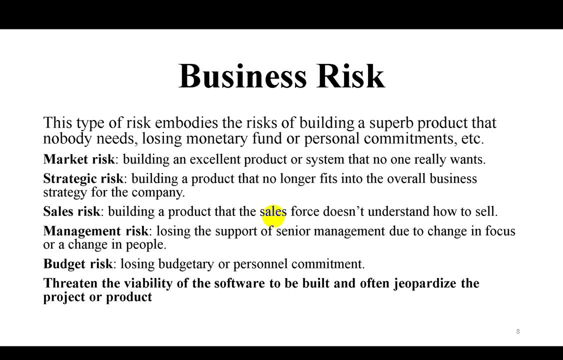 So we have to stop the overall project. We have to stop the project in between. The third type is the business risk. What is the business risk When a project is made and ready, the risks that will be there during the sale are also related to the business risk. 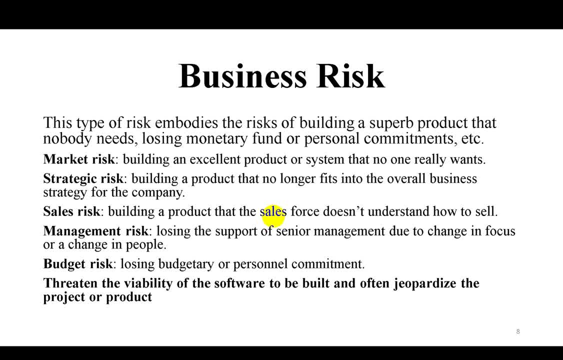 This type of risk embodies the risk of building a super product that nobody needs, losing monetary fund or personal commitments. What does this mean? We have made such a project, which is very good, but no one needs it, So this is a kind of business risk. 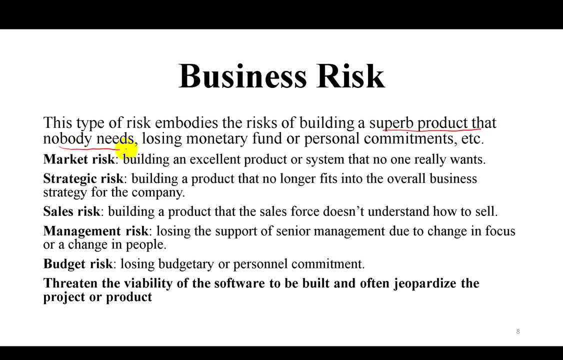 Superb product but nobody needs. No one needs it, Like losing monetary fund. What happened to us? The risk related to monetary or funding is also related to business risk, Personal commitment, The commitment that we have made, the agreement that has been made. 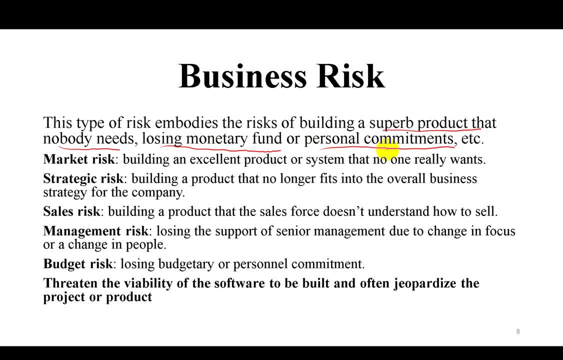 the commitment that was made by the customer and the developer. what are those risks related to business risk, If we talk briefly here. the first is the market risk. Market risk means that we have made such a product, which is excellent. It is excellent in itself. 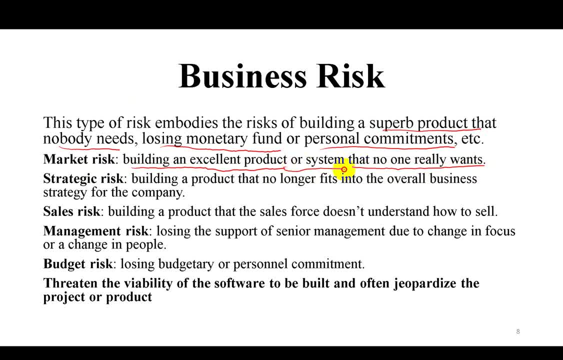 but no one really wants it, But no one needs it. Second one is strategic risk. What does strategic risk mean? Building a product that no longer fits with the overall business strategy for the company. For example, we have made such a product, which is MS-DOS based product, but in today's time, 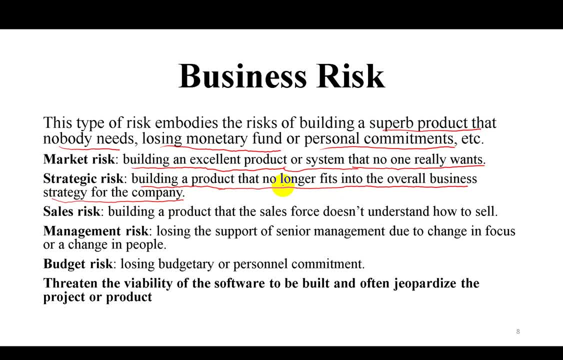 most of the companies are using MS-Windows or other operating system except for MS-DOS, so there it is not fitting according to the needs of those companies. so this is also a strategic risk, that building a product that no longer fits into the overall business strategy. 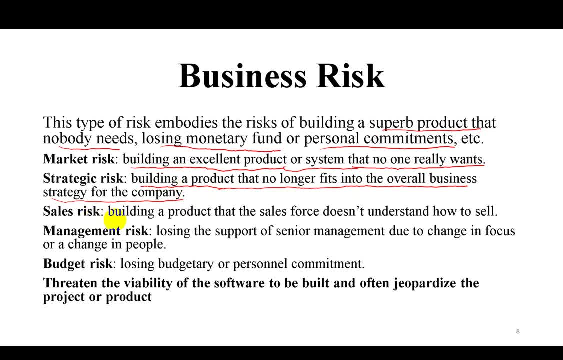 of the company. Third one: sales risk that the project which we have made and the sales team does not know how to sell that project- building a product that the sales force does not understand how to sell. this is also a business risk. 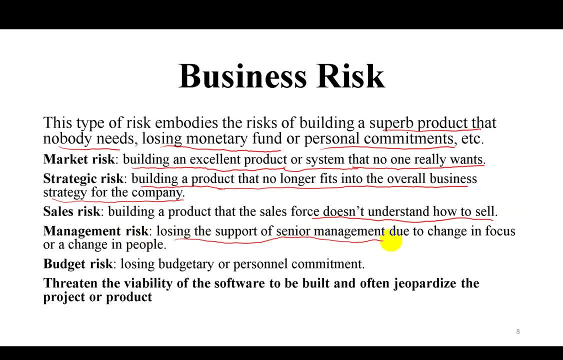 Management risk. what is the meaning of management risk? losing the support of senior management due to change in the focus or change in the people? what has happened in the top management of that project Change? If their focus has changed, then what is this? we also have a business risk that during 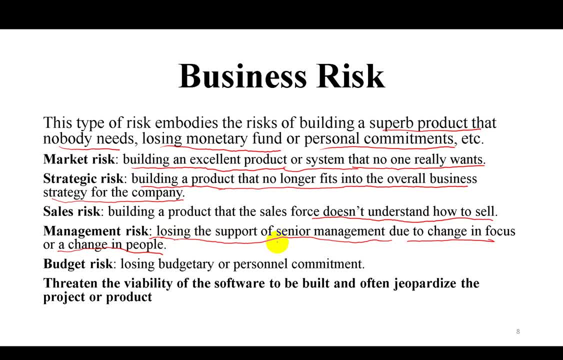 that time what we have to do? we have to drop that project in the middle Budget, risk losing budgetary and personal commitment that from where we had to have budget funding. it has been stopped. so this is also a business risk and what will be? 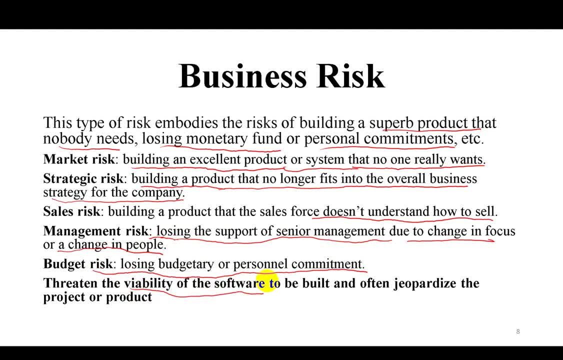 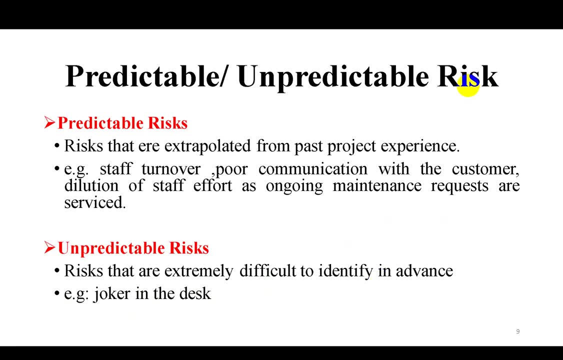 their effect threaten on the viability of the software to build and open, geopolitize the project or product. But what will happen to us due to this? It will have to stop the software in the middle. What is the category of predictable and unpredictable risk? 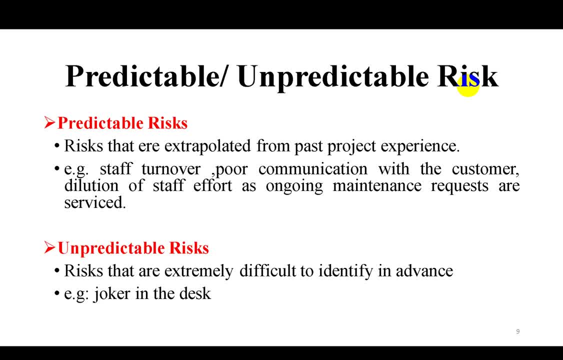 Predictable risk. we get the historical experiences from the old project we have already made, Based on the past experience. the risks that are identified we call predictable risk risks that are extrapolated from the past project experience, which are then distributed among the projects. 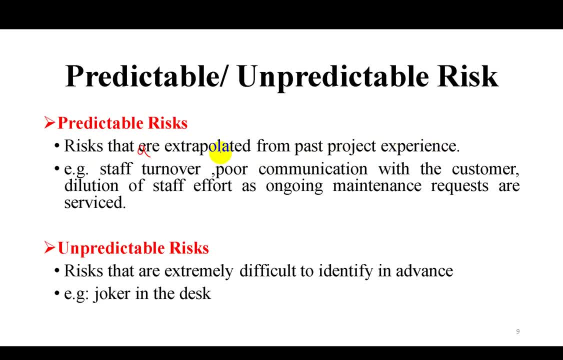 Those risks are predictable risks. Second point is predictable risks which we can extrapolate and estimate our past experiences. This is what we call Predictable Risk. For example, how many staff do we need for the turnover? Poor communication with the customer: If our communication was poor in an old project, we can improve it. 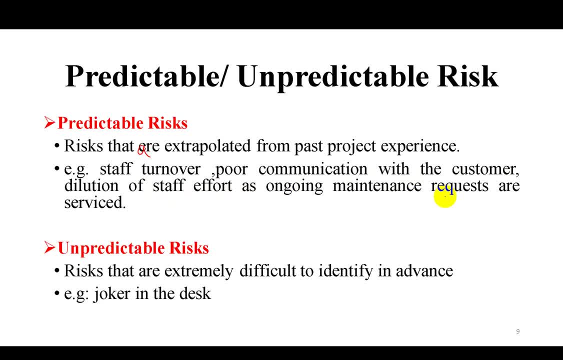 Dilution of staff effort, ongoing maintenance requests, etc. We can reduce the staff's team. What will be the effect in maintenance? These are the Predictable Risks And Unpredictable Risks. The Unforeseen Risks. The Unforeseen Risks: Risks that are extremely difficult to identify in advance. 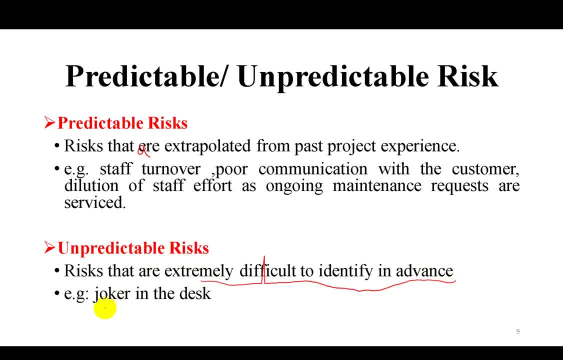 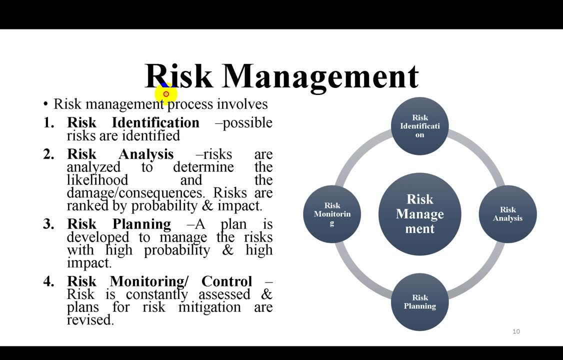 These are called Unpredictable Risks. For example, Joker in a Dusk. This is a very famous idiom. It means that we don't know when we will be cheated, So These are called Unpredictable Risks. After that we will discuss about Risk Management. 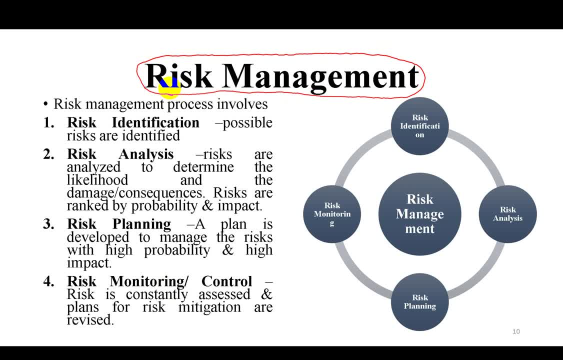 What is Risk Management? Risk Management is an overall process In which we have many steps. The combination of all these steps is called Risk Management. The four main steps in Risk Management are: Risk Identification. The first step is: First of all, we have to identify the risk. 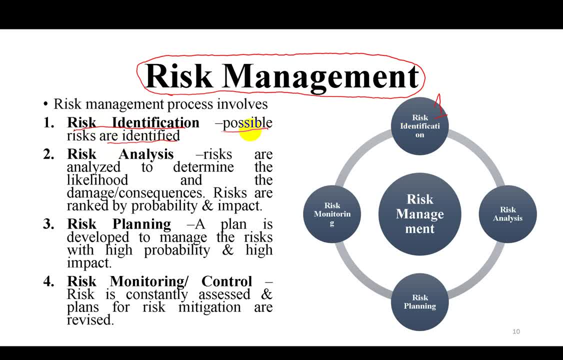 Which risks can be. We will identify the Predictable Risks. Second, we will analyze the risk. We will analyze the risk that we have identified. Which risk is affecting us more? Which is reducing our project? Whose probability is more? Whose probability is less? Based on that, we rank the risk. 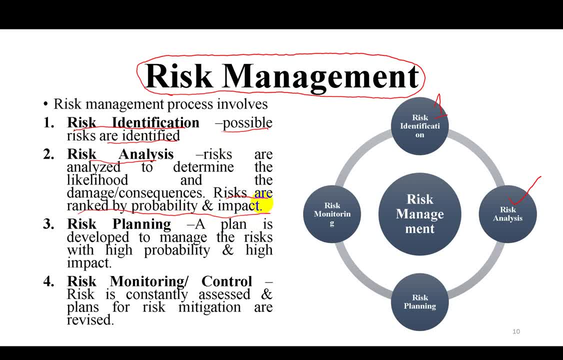 Based on their probability and impact. Third one: Risk Planning. What will happen in Risk Planning? We will have a plan How to handle those risks Or how to avoid them. It is known as Risk Planning. It is a planning to manage the risk With high probability and high impact. 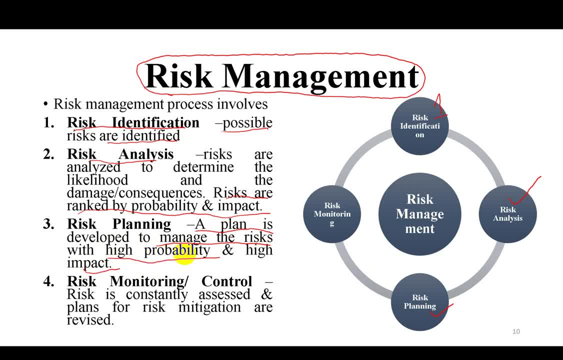 The risk, which is high probabilistic And high impact. The way to manage the cost on the staff or schedule Is known as Risk Planning. Next is Risk Monitoring and Control. In Risk Monitoring, if we have the risk, We constantly assess our project And in between we avoid the risk. 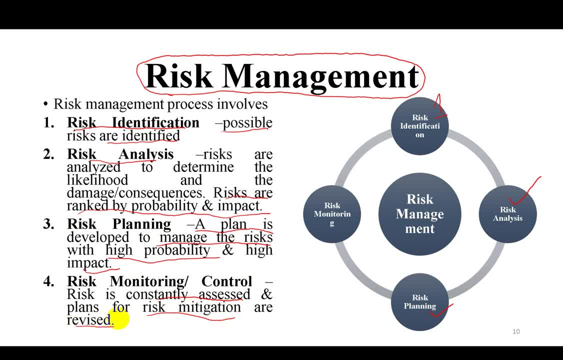 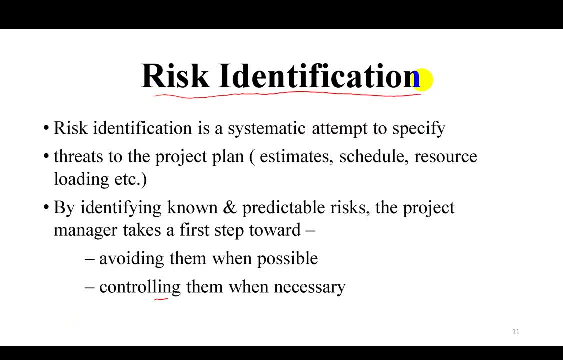 And revise our process That is known as Risk Monitoring and Control. First of all, we have Risk Identification. So what is Risk Identification? It is a systematic attempt to specify threats to the project, This systematic way of identifying threats Which affects our software project, In which we estimate: 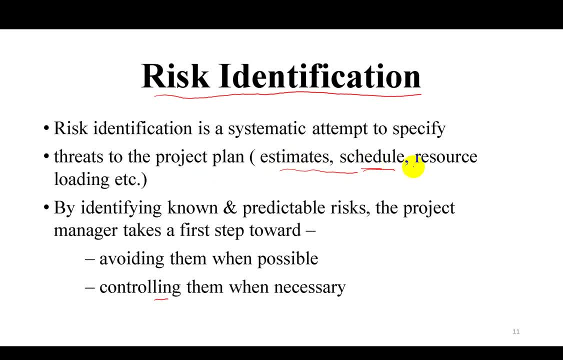 Schedule: Estimate of cost. Estimate the schedule. What will be the resources? In this way, we can identify the risks In a systematic way. By identifying known and predictable risks, The project manager takes the first step towards On the basis of these risks Which we have identified. So what will the project manager do? 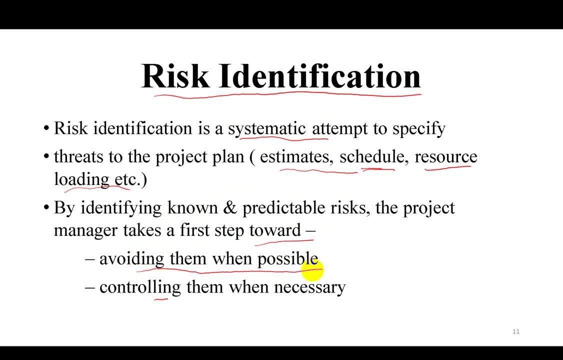 Either he will avoid them, He will do the planning to avoid them, How to avoid the chances of those risks, And if it cannot be avoided, Then how to control them. Which will be affected by them. That is known as Risk Monitoring and Control. That can be done with the help of Risk Identification. 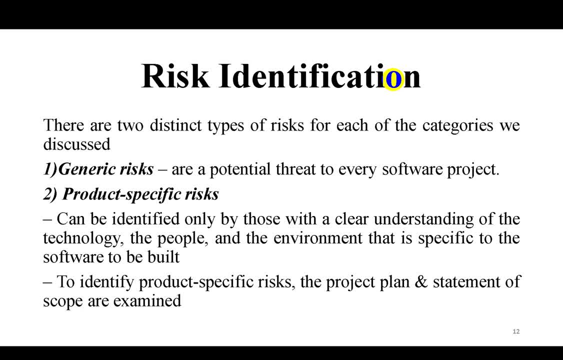 There are two types of risks for each category. There are two types of risks: Generic risks, Which are potential threats to every software project, Which generally come in every project, And the second type is Product specific risks, Which are related to that specific project. These can be identified only by those. 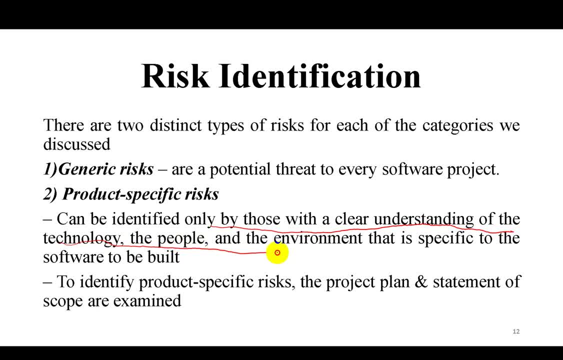 Who have a clear understanding of the technology, The people and the environment That is specific to the software to be built. It is comparatively easy to identify the generic risks, But to identify the product specific risks Is difficult as compared to generic risks. Why? Because for this we need specific people. 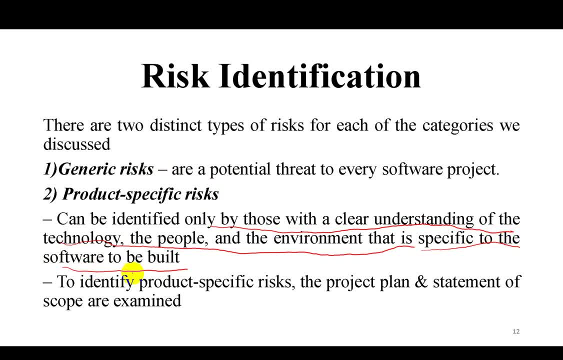 Who have already worked in that type of environment To identify product specific risks. The product specific risks, The project plan and statements Have to be examined. Once they are identified, We examine the planning of the project, How we have to plan to implement that project. Now what are the methods to identify the risk? 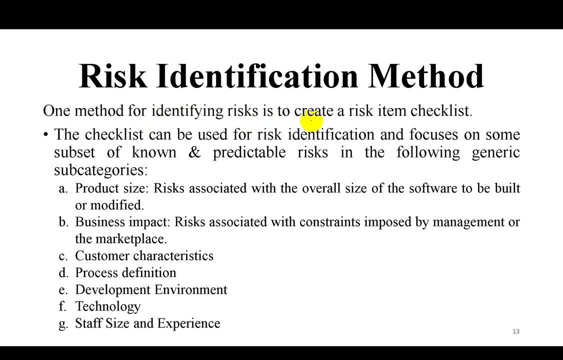 One of the methods for identifying risk Is to create a risk item checklist. What we do is We make a checklist of the risks that can come And, based on that checklist, We rank them. So what is the first thing? A checklist can be used for risk identification And focuses on some subset of known and predictable risks. 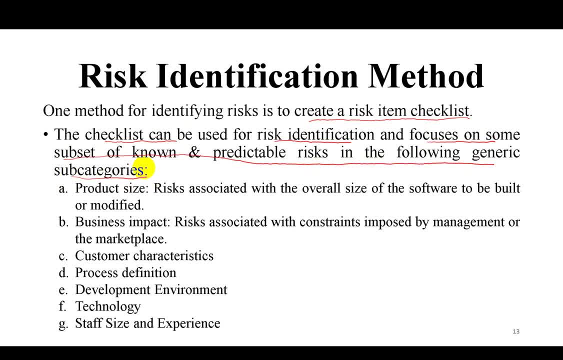 In the following generic subcategories We make a checklist of the predictable risks, For example, product size. What will be the risk in this? The risk will be related to the size of the product, The risk associated with the overall size of the project To be built or modified. 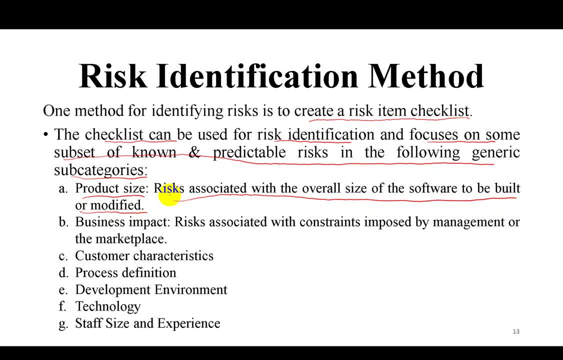 So all the risks related to this. We will identify them here. Second, business impact. Such risks that will affect the business Risk associated with the Constraints imposed by management or the market place. What are the constraints imposed by the management Or when we go to sell it in the market? 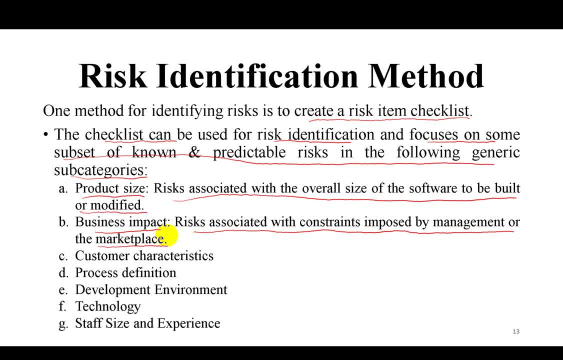 Then what will be the conditions? So the risks related to them Will be related to business impact. Third, customer characteristics. What are the requirements of the customers? Which process we have to use, In which environment or technology Based on which we have to make our project? What will be the size of our team? 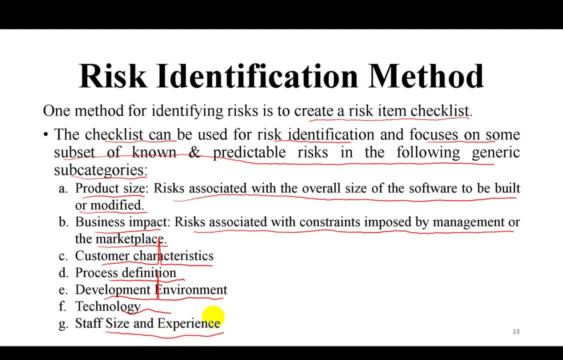 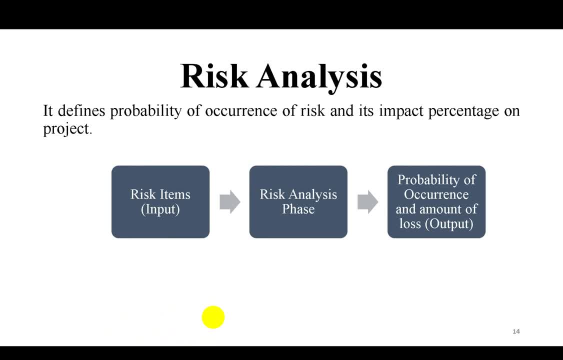 And what will be the experience of that team? On the basis of that, We make a checklist of the risks And after making this checklist, We will do the second phase, Risk analysis. So what happens in risk analysis? Based on the checklist made, On the basis of that, We will check the probability of occurrence of risk. 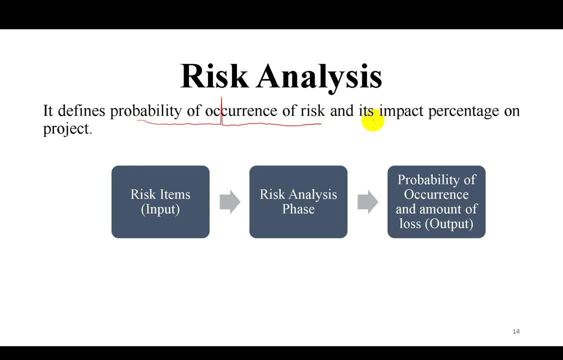 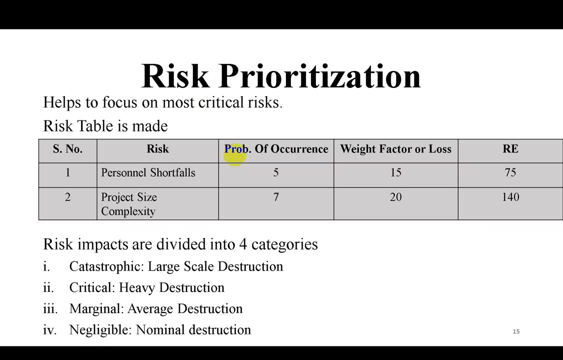 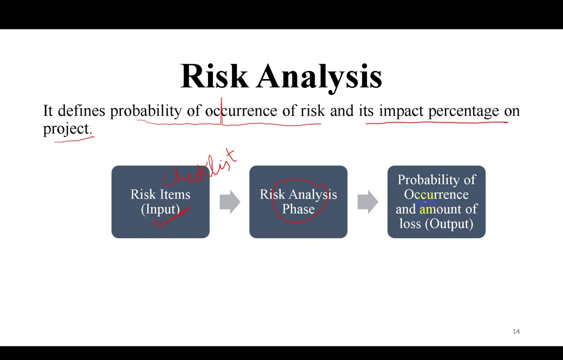 And the chances of that risk And as well as their impact Percentage of the project. So in the risk analysis phase We have basically input, Risk items, Which we have made, the checklist. We have made the checklist And what will be its output: Probability of occurrence of the risk. 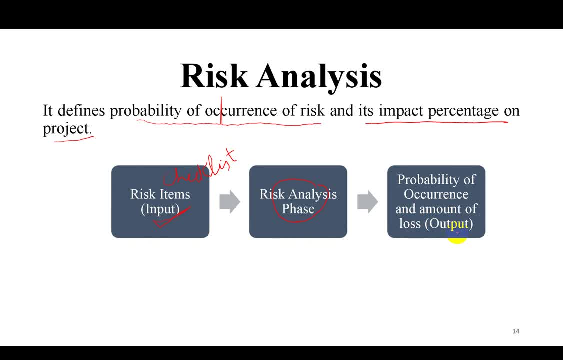 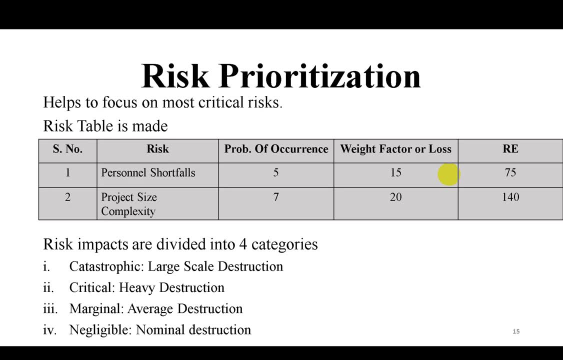 As well as the amount of the loss That happened due to that risk. So these two things Will give us the output. So what we will do in risk analysis? First of all, We will prioritize the risks that have come. Which risk has more effect? Which risk has less effect? 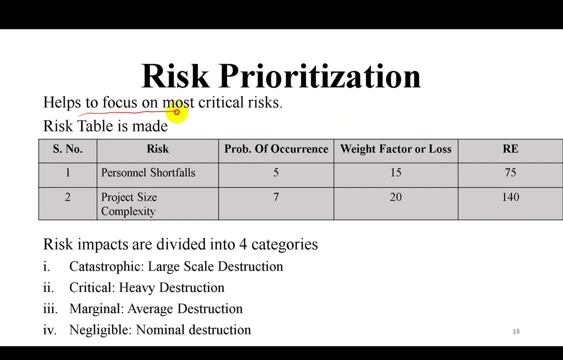 Like our IT, Helps us to focus on most critical risk, So that we don't emphasize all the risks And the most critical risk Which we can concentrate on them. So the risk table will be like this: One of the example of the risk table Is serial number, The name of the type of risk. 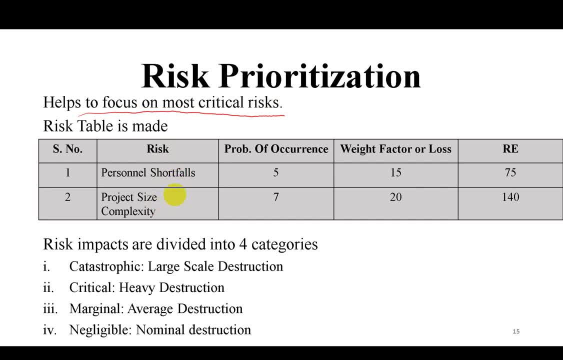 Like personal shortfalls, Project size, complexity. We will calculate the probability of that. How much impact will it have on the weight factor? We will calculate that And after that we will calculate its risk RE factor, Which will multiply the two Like 5x15, 7x20. 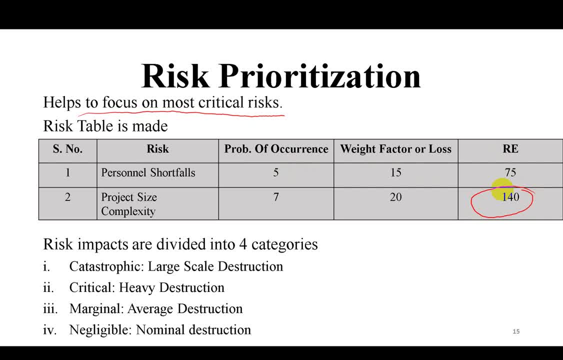 So, on the basis of this, This risk is more critical, So we will give more emphasis to this. To handle as compared to this risk. So it is the table for risk prioritization. Risk impacts are divided into the four categories. So, on the basis of that, We divide the risk into four categories. 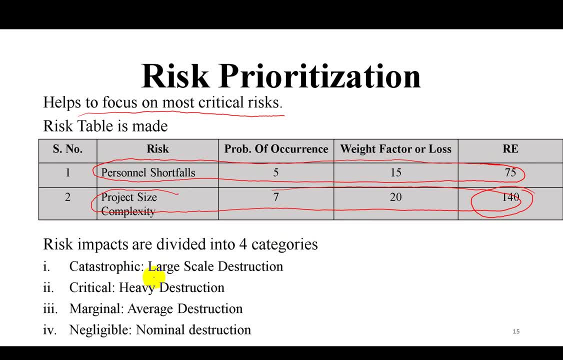 First is catastrophic risk, From which we have a lot of effect: Large scale destruction Which will affect our system or project very heavily, So we have to handle them. After that comes critical risk Which will do less harm than them But again do a heavy destruction. Third one is the marginal. 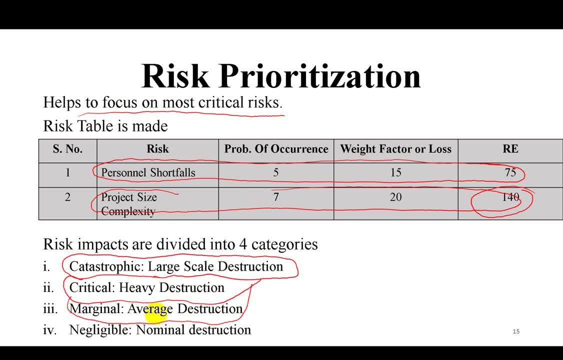 From which we have Marginal risk, From which we have an average effect on our system, Which is the average destruction, And we can avoid the negligible risk, From which we have an average effect on our system, Which means Negligible or nominal destruction Which affects our system. 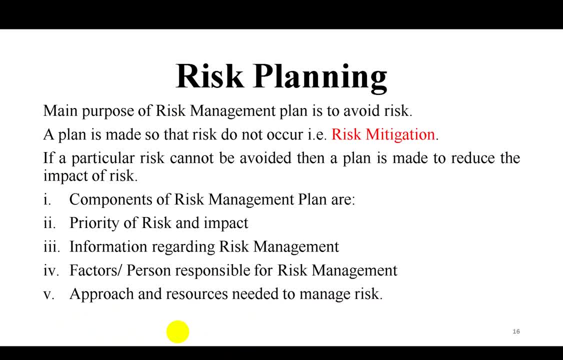 And fourth one, Sorry. The third step in risk management Is risk planning. So what is risk planning? Basically, we call risk planning as risk mitigation. What is the meaning of risk mitigation? That the risk does not happen. So in risk planning, What we generally do is The main purpose of the risk management plan. 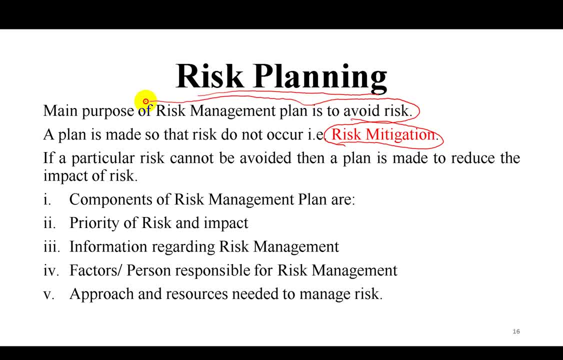 Is to avoid the risk Doing such planning, Because of which the risk does not happen. That kind of planning is called risk planning phase. A plan is made so that the risk does not occur. So this is what we call risk mitigation: If a particular risk cannot be avoided. 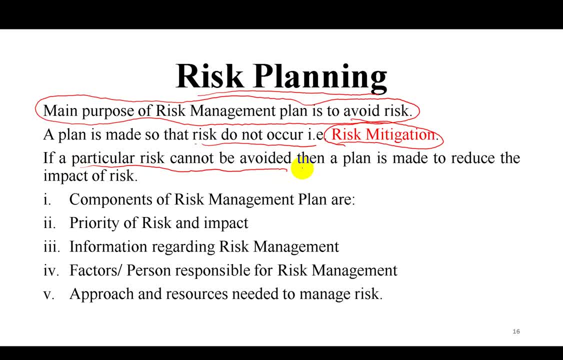 And sometimes it happens that We cannot avoid any risk. So in that case What we will do is We will make such a plan So that the impact of the risk we have Will be reduced. So what will happen in risk planning? We will make such a plan So that the risk does not happen. 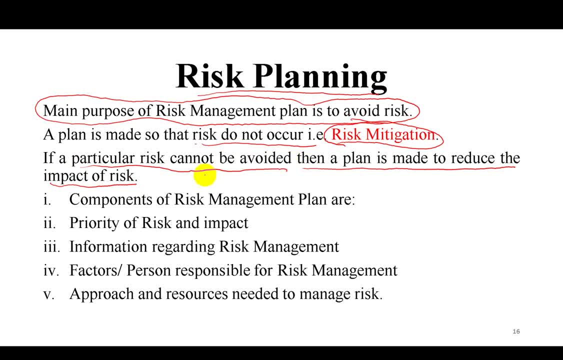 And if it happens, Then its impact will be minimal. The components of the risk management plan: What are its components? Priority of the risk and their impact. Information regarding them. Risk management Factors or person risk management. Responsible for the risk management. Approaches and resources needed for the risk management. 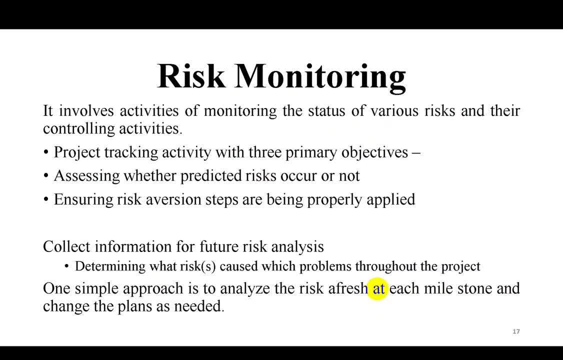 So yeah, This is the risk planning phase And the last one Is the risk monitoring phase. So we have the risk monitoring phase. Risk monitoring phase is When we have done risk planning. We have avoided some risks, But some risks cannot be avoided. So in that case, When we are implementing the project, 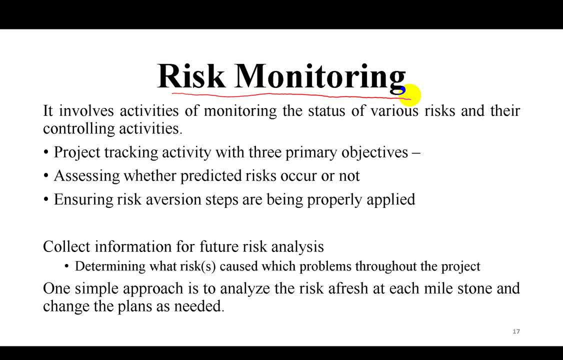 We are monitoring the risk And on the basis of that We change our plan, We update it So that the effect of the risk Can be minimized. And if there is an unpredictable risk, Then what is its strategy So that its effect can be minimized? It is all the process of the risk monitoring. 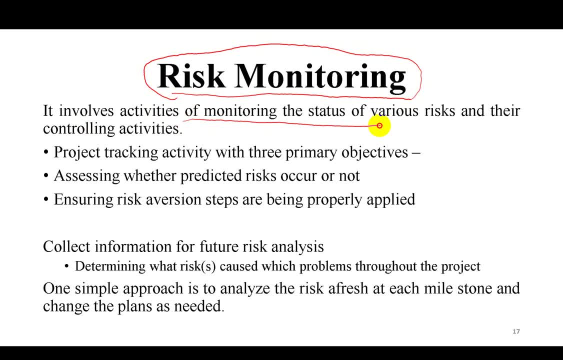 It involves the activities of monitoring The status of various risks And their controlling activities. So what we do here? We analyze every risk, We update about their status And on the basis of that We change our strategic plan. It involves project tracking activity With three primary objectives. Number one: 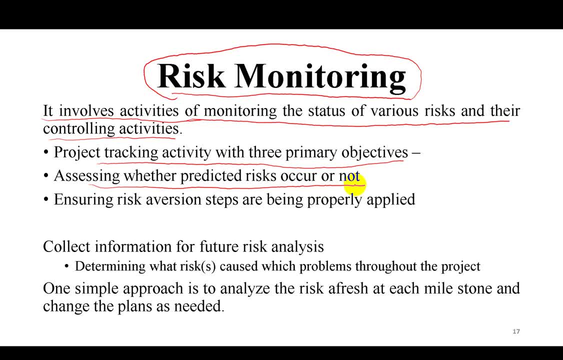 Assessing whether the predictable risk Happens or not. So, first of all, we see that, Whether the risk has happened Or not, Second, Ensuring risk aversion steps Are being properly applied In the sense of risk aversion. The steps to remove the risk Have been applied easily. 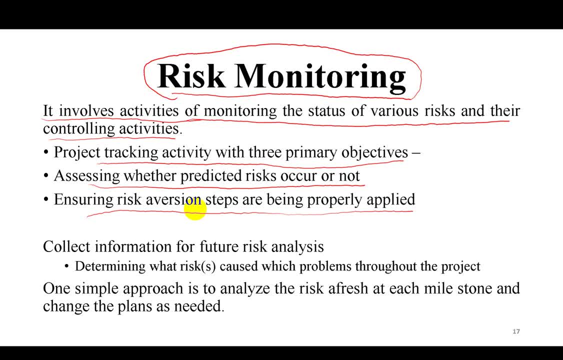 Or not. One of the most important part of this Is to collect information For the future risk analysis. So what we do here: Determine which risks Caused which problems Throughout the project. On the basis of these, We keep a proper information So that we can handle those risks.